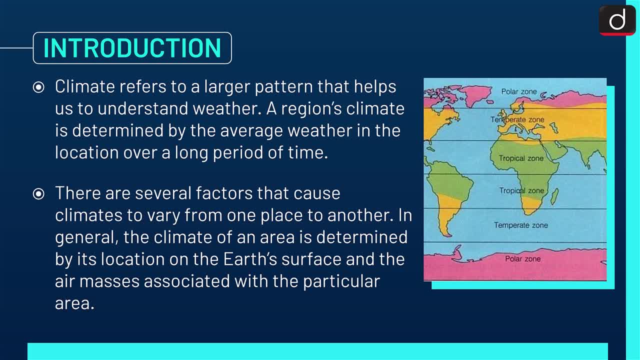 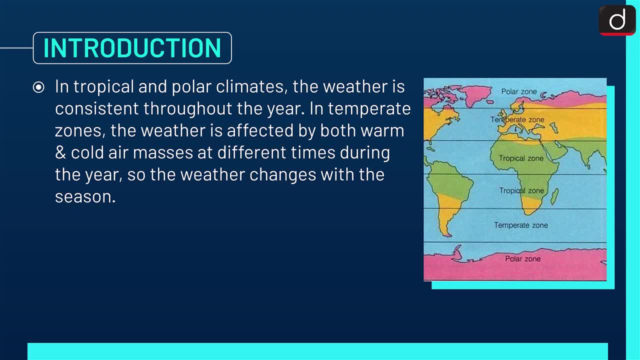 air masses associated with the particular area. In tropical and polar climates, the weather is consistent throughout the year. In temperate zones, the weather is affected by both warm and cold air masses at different times during the year, So the weather changes with the seasons. 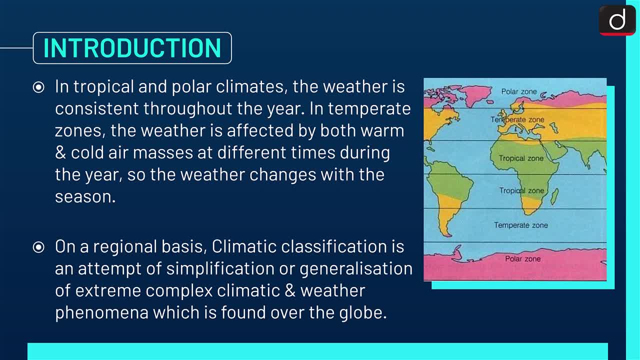 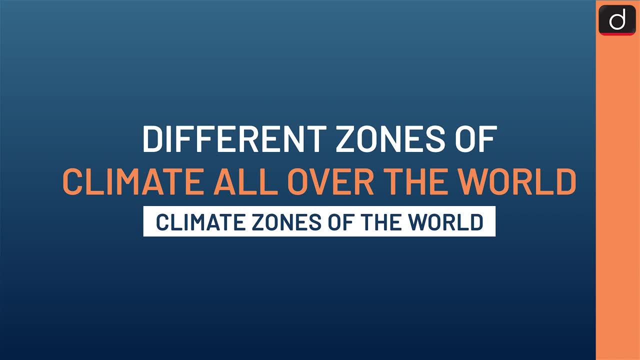 On a regional basis. climatic classification is an attempt of simplification or generalization of extreme, complex climatic and weather phenomena which is found over the globe. Now let's discuss about different zones of climate all over the world. First is the hot-wet equator. 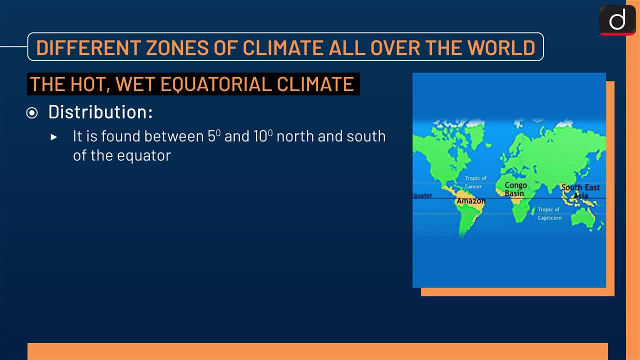 Now moving to the distribution. first, It is found between 5° and 10° north and south of the equator. It is dominantly found in the lowlands of the Amazon, the Congo, Malaysia and the East Indies. Next is climate. There is great uniformity of temperature throughout the year. The mean 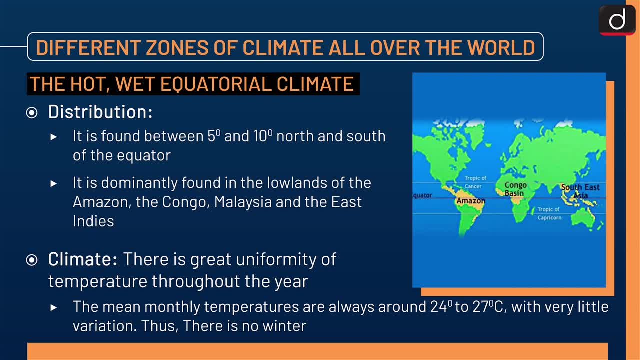 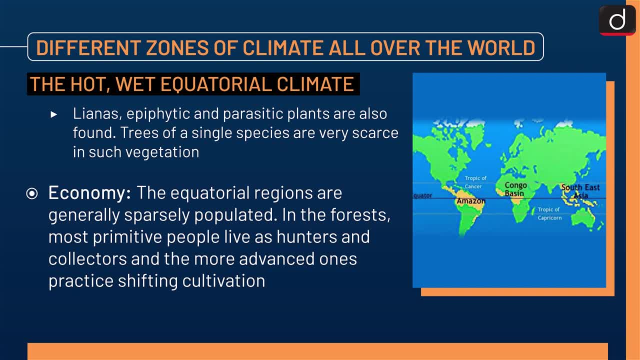 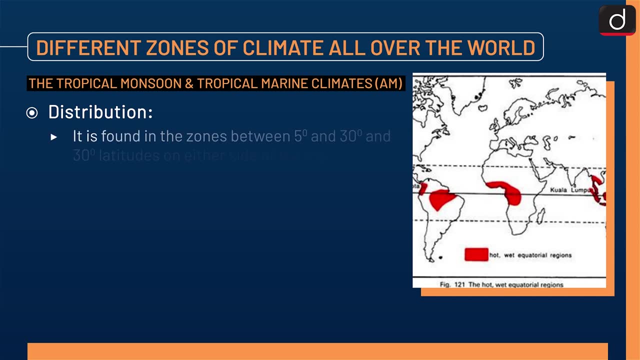 The equatorial regions are generally sparsely populated. In the forest, most primitive people live as hunters and collectors, and the more advanced ones practice shifting cultivation. Now, next zone is the Tropical Monsoon and Tropical Marine Climates distribution It is found in the zones between 5° and 30° and 30° latitudes on either side of the equator. 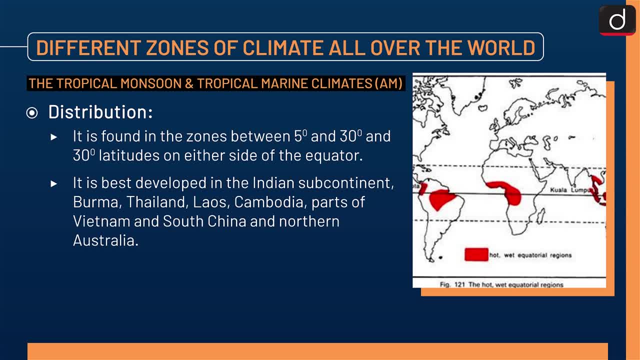 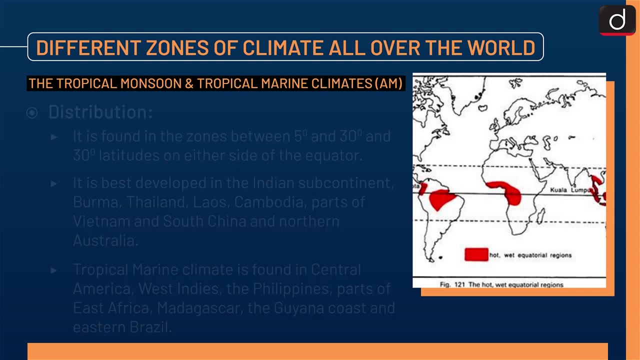 It is best developed in the Indian subcontinent, Burma, Thailand, Laos, Cambodia, parts of Vietnam and South China and Northern Australia. Tropical marine climate is found in Central America, West Indies, the Philippines, parts of East Africa, Madagascar, the Guana coast and Eastern Brazil. 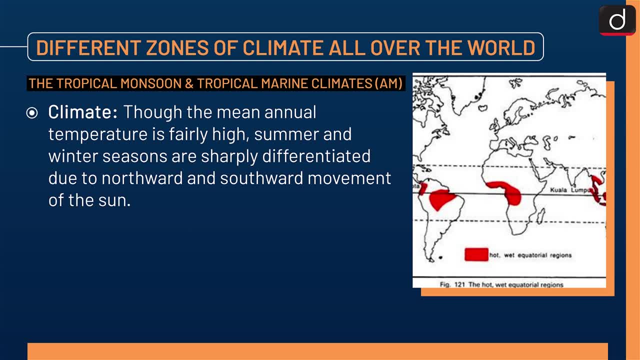 Next is climate. Though the mean annual temperature is fairly high, Summer and winter seasons are sharply differentiated due to northward and southward movement of the sun. Average temperature of warm, dry summer months ranges between 27°C and 32°C. Most of their annual rainfall occurs through cyclonic and orographic types of rain. 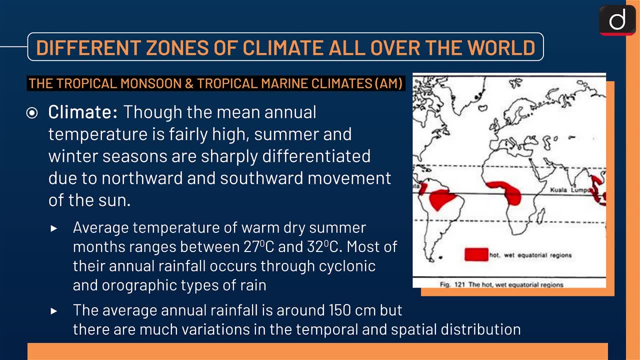 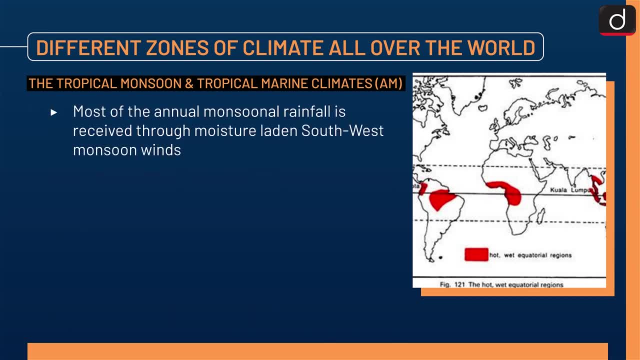 The average annual rainfall is around 150 cm, but there are much variations in the temporal and spatial distribution. Most of the annual monsoonal rainfall is received through moisture-laden south-west monsoon winds. Next is natural vegetation: Trees are normally deciduous. 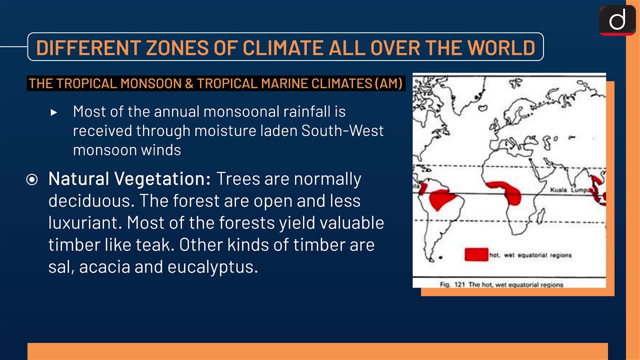 The forests are open and less luxuriant. Most of the forests yield valuable timber-like tea. Other kinds of timber are saal, acacia and eucalyptus. Economy, People are mainly engaged in agriculture, Agri-culture. 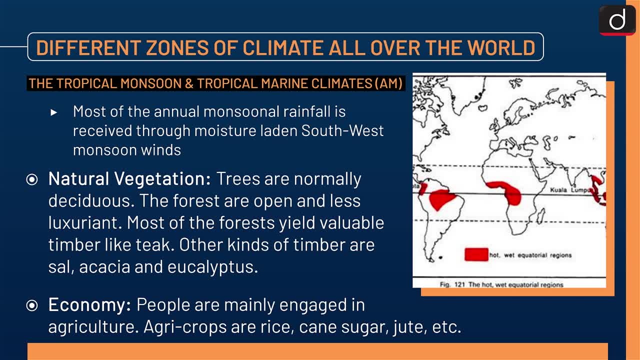 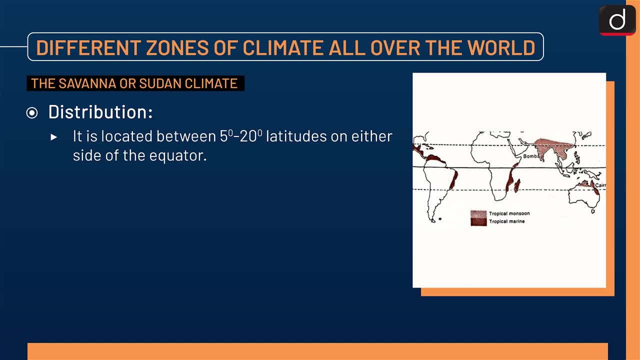 Agri-crops are rice, cane, sugar, jute, etc. Next zone is the savanna, or sudan climate distribution. It is located between 5 inches to 20 inches latitudes on either side of the equator. It is transitional type of climate found between the equatorial forest and the semi-arid, and 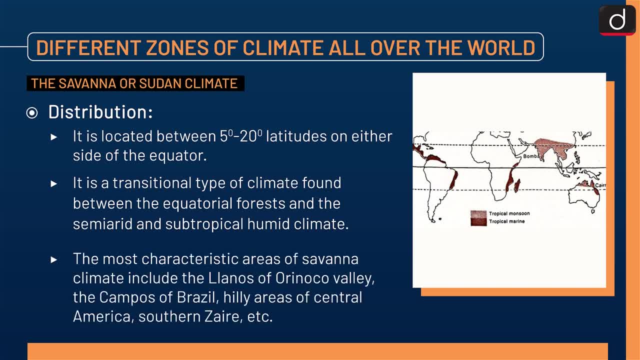 sub-tropical humid climate. The most characteristic areas of savanna climate include: The most characteristic areas of savanna climate include The Llanos of Orinoco Valley, the Campos of Brazil, hilly areas of Central America, southern Zaire, etc. 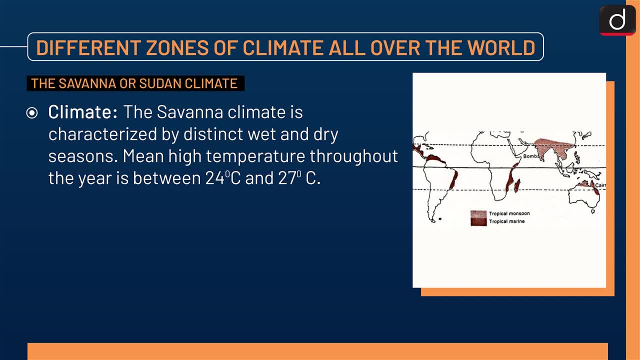 Climate. The savanna climate is characterized by distinct wet and dry seasons. Mean high temperature throughout the year is between 24 degree C and 27 degree C. The annual range of temperature is between 3 degree C and 8 degree C. Cold thermes, weak airによる Kirschац and Pl Gavinоз in the winter. 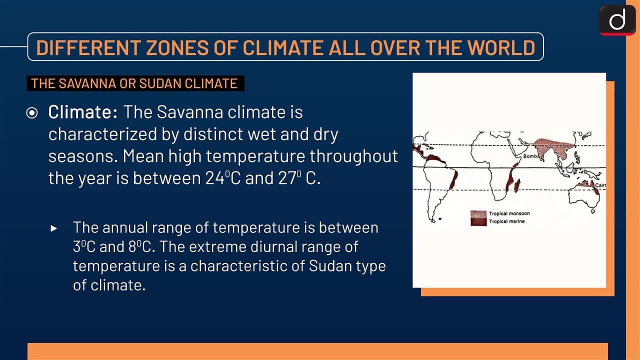 This nuestros climate is understood as a natural graduate of Trinidad and Tobago. The climate is realized by climate and constant low-frontalede. remember our natural climate, Whatutt Celsius. the extreme diurnal range of temperature is a characteristic of Sudan type of climate and the average annual rainfall ranges between 100. 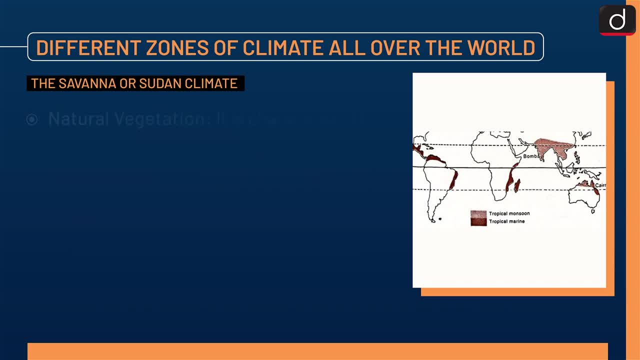 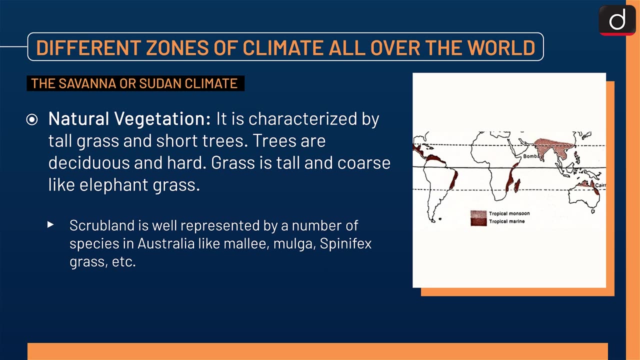 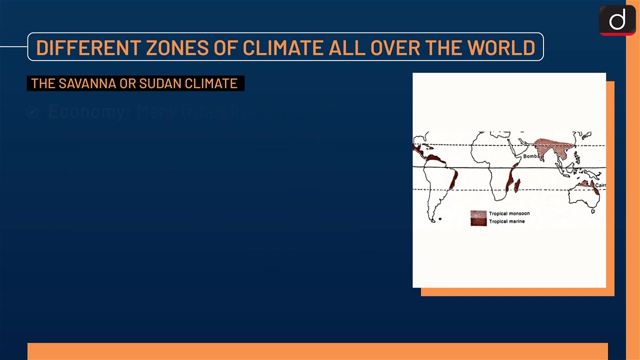 centimeter and 150 centimeter natural vegetation. it is characterized by tall grass and short trees. trees are deciduous and hard grass is tall and coarse, like elephant grass. scrubland is well represented by a number of species in Australia, like Mali Mulga, spinifex grass, etc. economy: many tribes live. 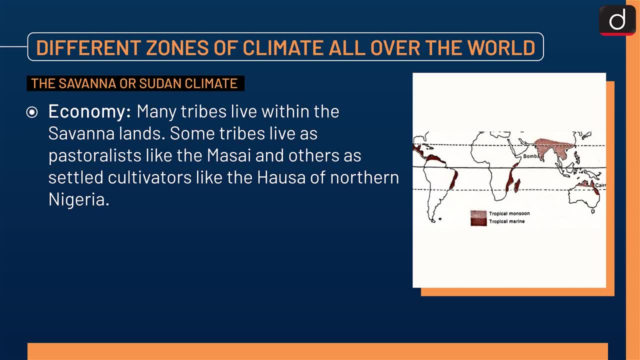 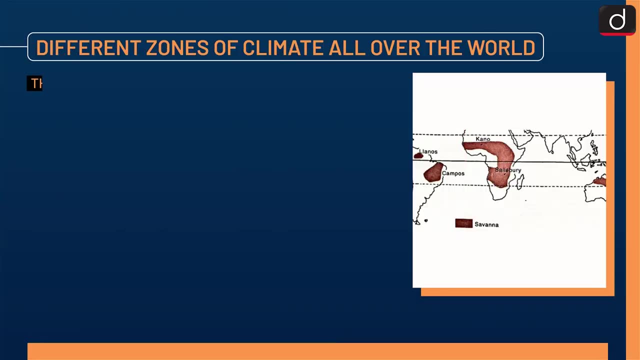 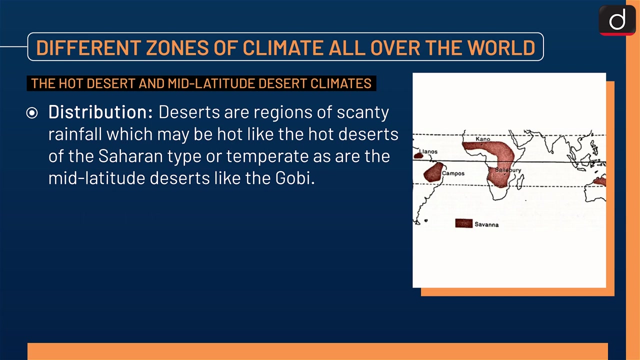 within the savannah lands. some tribes live as pastoralists, like the Maasai, and others as settled cultivators, like the Hausa of northern Nigeria. however, agriculture is not much developed. next zone is the hot desert and mid-latitude desert climate. moving on to the distribution, first deserts are regions of scanty rainfall. 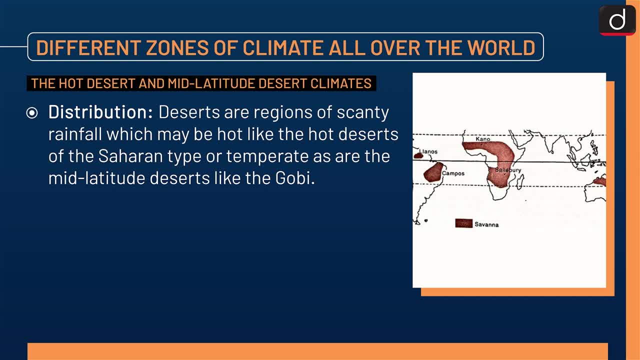 which may be hot, like the hot deserts of the Saharan type, or temperate, as are the mid-latitude deserts like the Gobi. the major hot deserts of the world are located on the western coast of continents between latitudes 15 degree. 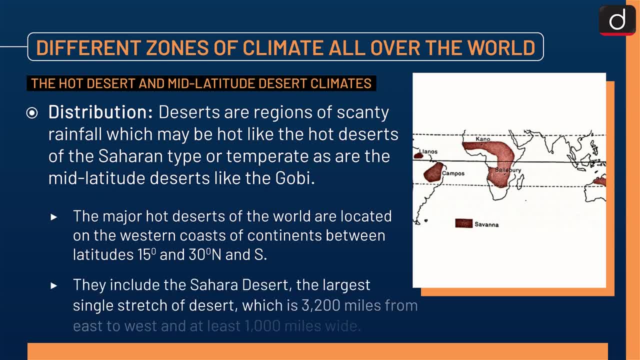 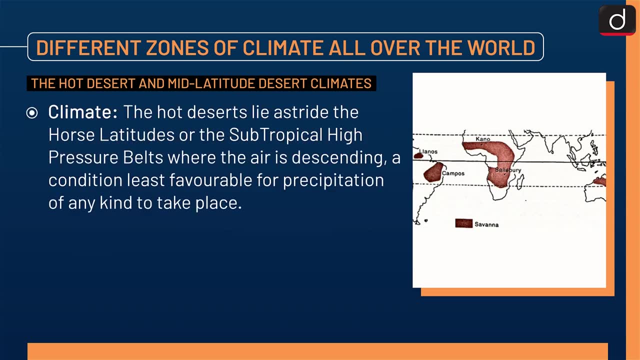 and 30 degree north and south. they include the Sahara Desert, the largest single stretch of desert, which is three thousand hundred miles from east to west and at least 1,000 miles wide. next is climate. the hot deserts lie astride, the horse latitudes or the subtropical high. 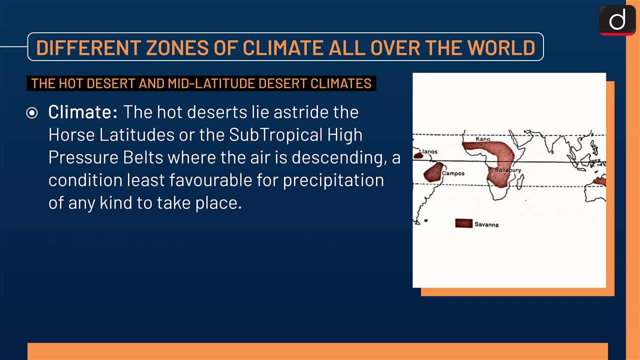 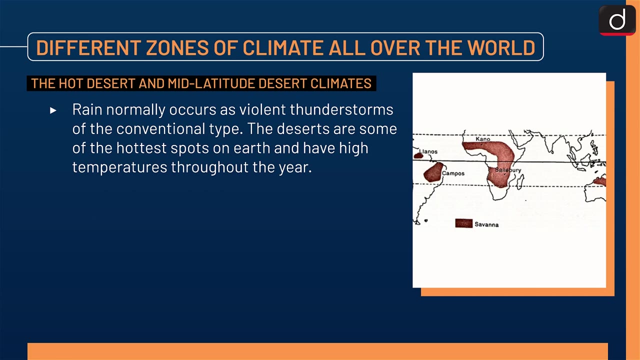 pressure belts where the air is descending, a condition least favorable for precipitation of any kind to take place. the relative humidity is extremely low, decreasing from sixty percent in coastal districts to less than thirty percent in the desert ins jotka and normally occurs as violent under storms of the conventionals지만 of the hottest sports on earth, and as high. 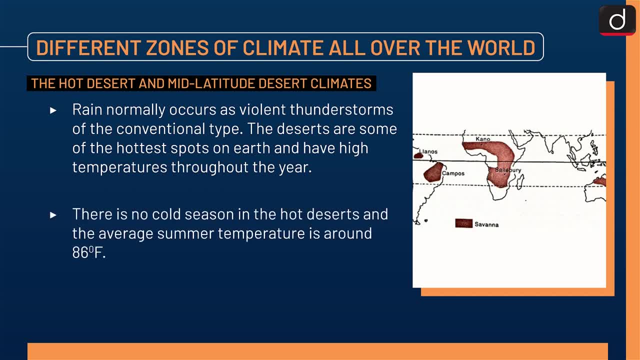 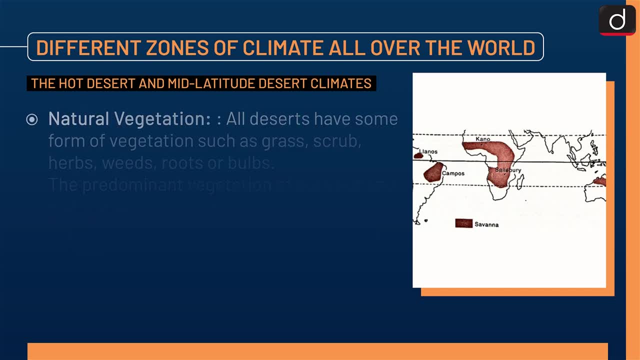 temperatures throughout the year. there is no season in hot deserts and average summer temperature around it is 6 degrees Fahrenheit. colors the next have some form of presentation, such as grass. perto help leads root. The predominant vegetation of both hot and mid-latitude deserts is xerophytic or drought-resistant. 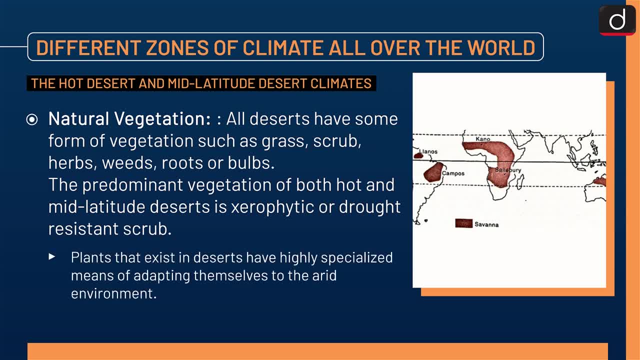 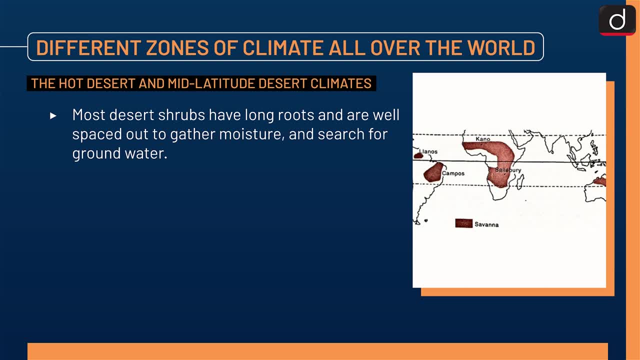 scrub Plants that exist in deserts have highly specialized means of adapting themselves to the arid environment. Most desert shrubs have long roots and are well spaced out. to gather moisture and search for groundwater, Plants have few or no leaves, and the foliage is either waxy, leathery, hairy or needle-shaped. 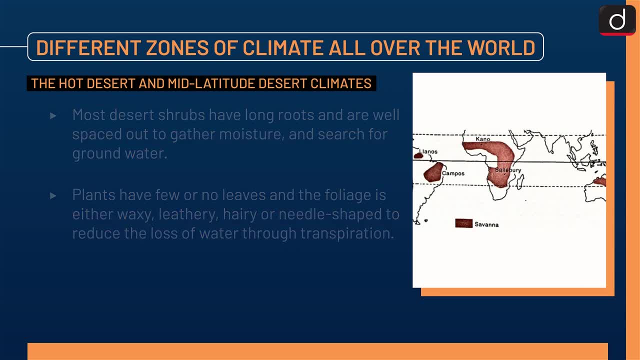 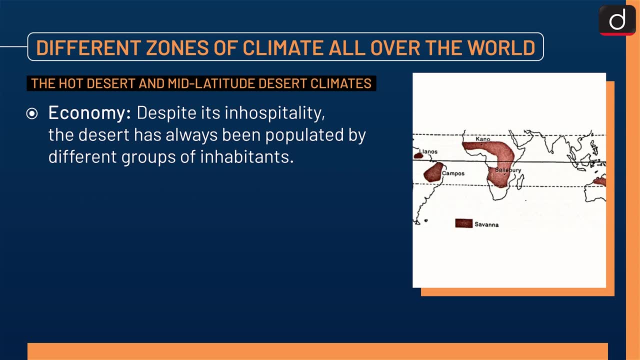 to reduce the loss of water through transpiration. Next is Economy. Despite its inhospitality, the desert has always been populated by different groups of inhabitants. Some, like the Egyptians, have attained a high level of civilizations. Others, like the Bedouin Arabs, have fared quite well with their flocks of sheep, goats, camels. 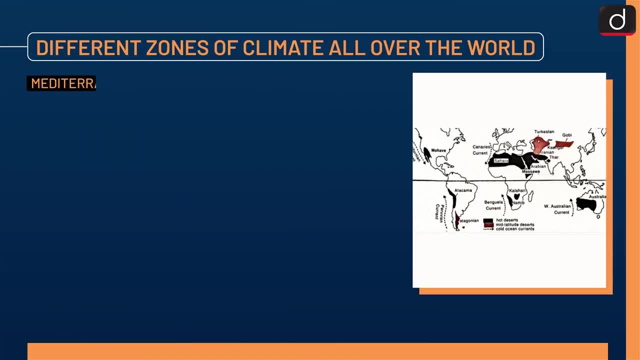 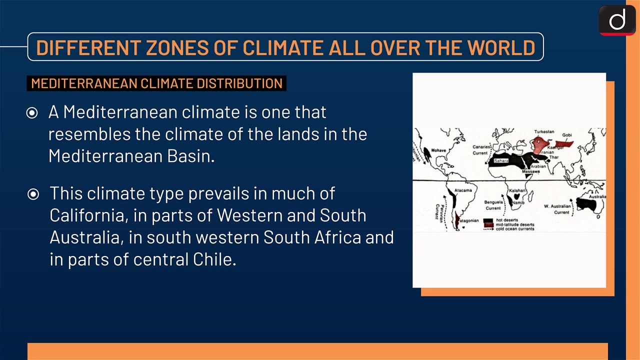 and horses. Mediterranean Climate Distribution. A Mediterranean climate is one that resembles the climate of the lands in the Mediterranean basin. This climate tribe prevails in much of California, in parts of Western and South Australia, in southwestern South Africa and in parts of central Chile. 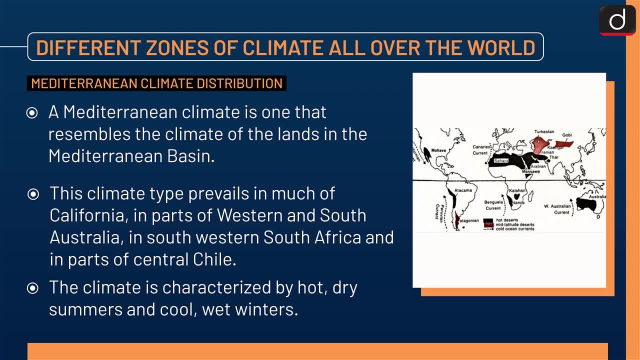 The climate is characterized by hot, dry summers and cool, wet winters. In the first three-degrees, the climate is characterized by a hot, dry summer and cool, wet winters. The climate is characterized by a hot, dry summer and cool, wet winters. 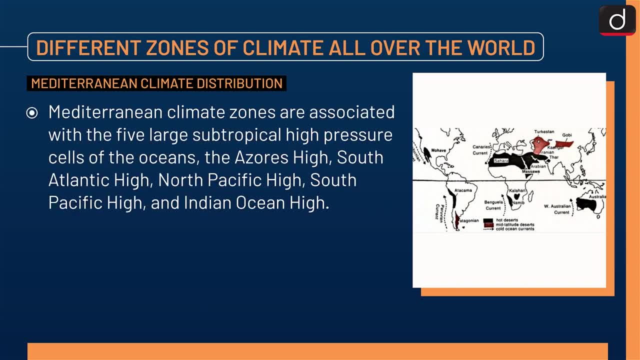 Mediterranean climate zones are associated with the five large subtropical high-pressure cells of the oceans: the Azores High, South Atlantic High, North Pacific, High South Pacific High and Indian Ocean High. Next is climate. All regions with Mediterranean climates have relatively mild winters, but summer temperatures. 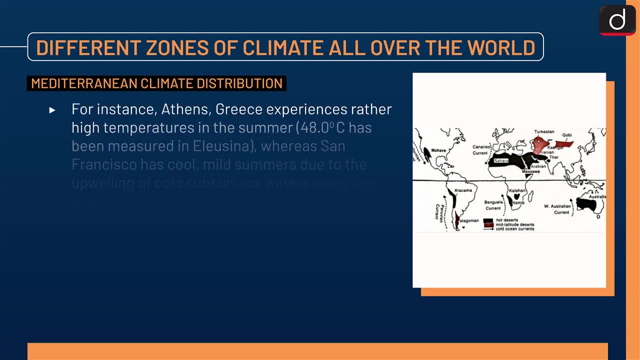 are variable depending on the region. For instance, Athens, Greece, experience rather high temperatures in the summer, ie 48.0 °C has been measured in Eleusina, whereas San Francisco has cool, mild summers due to the upwelling of cold subsurface waters along the coast. 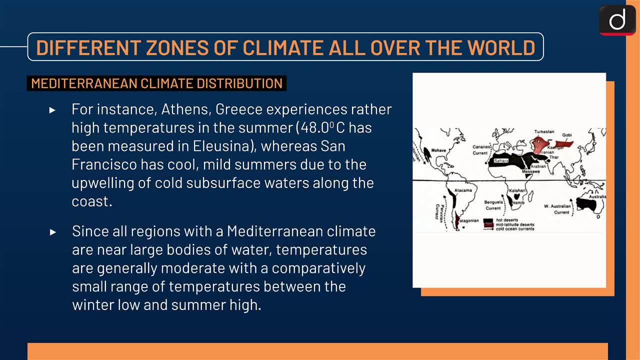 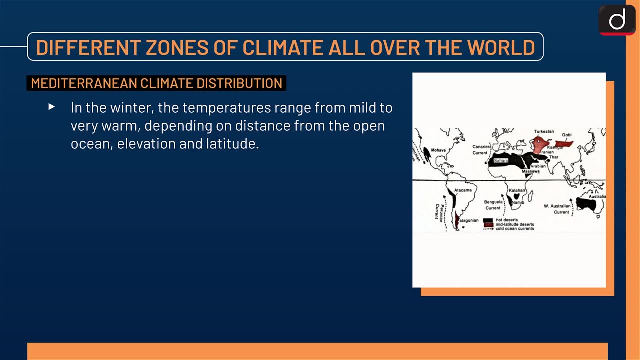 Since all regions with a Mediterranean climate are near large bodies of water, temperatures are generally moderate, with a comparatively small range of temperatures between 10 to 15 °C between the winter low and summer high. In the winter the temperatures range from mild to very warm, depending on distance from. 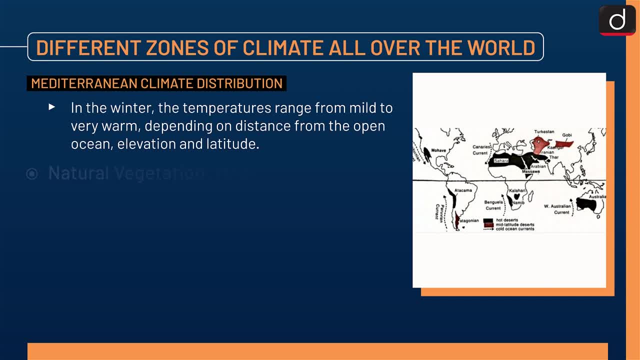 the open ocean, elevation and latitude. Next is natural vegetation. Mediterranean vegetation includes the following Evergreen trees such as cork, oak and eucalyptus, jaraha and kari. in Australia, Evergreen coniferous trees are pines, firs, cedars and cedars. Evergreen coniferous trees are pines, firs, cedars and cedars. Evergreen coniferous trees are pines, firs, cedars, cedars and cedars. Evergreen coniferous trees are pines, firs, cedars, cedars and cedars. 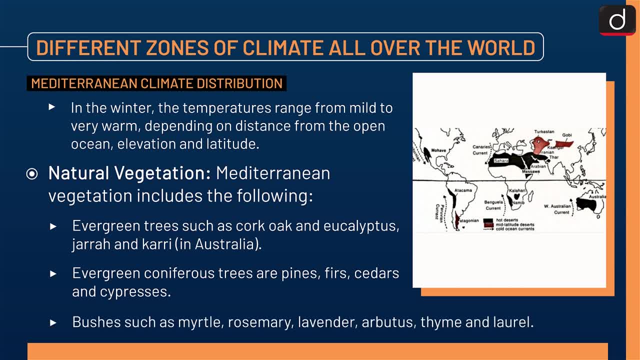 Evergreen coniferous trees are pines, firs, cedars and cedars. Evergreen coniferous trees are pines, firs, cedars and cedars, Bushes such as miretar, rosemary, lavender, arbutus, thyme and laurel. 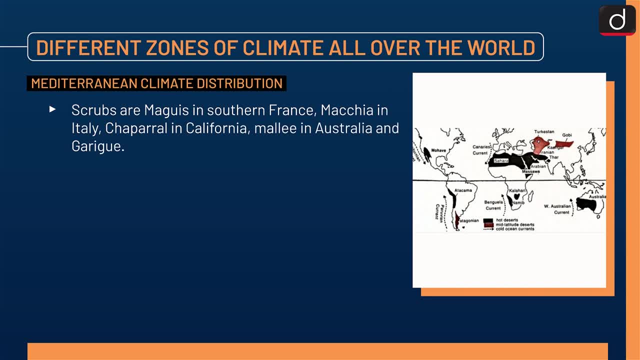 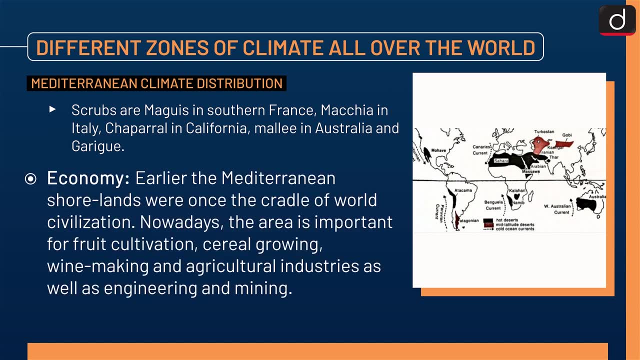 Scrubs are maegios in southern France, Maikia in Italy, chaparral in California, Mali in Australia and Gharifi. Next is economy. Earlier, the Mediterranean shore lands were once the cradle of world civilization. Nowadays, the area is important for fruit cultivation. 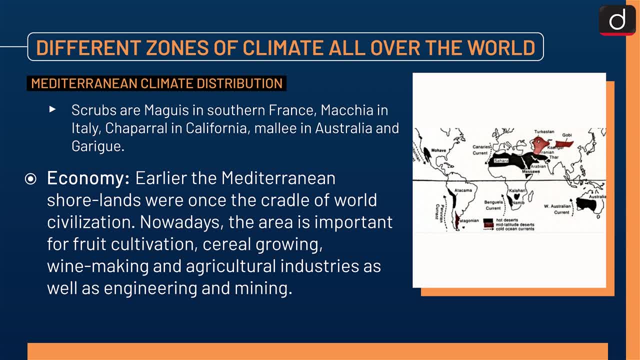 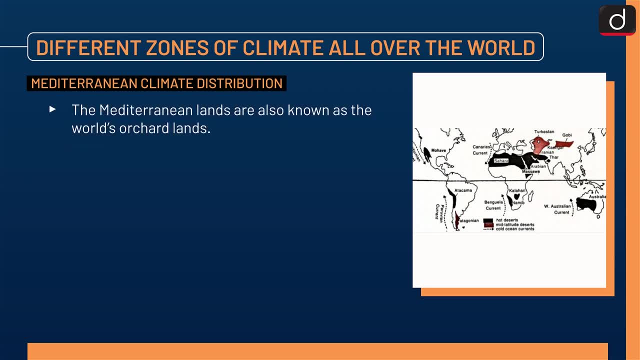 cereal growing, winemaking and agricultural industries, as well as engineering and mining. the mediterranean lands are also known as the world's orchard lands. the mediterranean lands account for 70 percent of the world's exports of citrus fruits. cereals are also grown in the 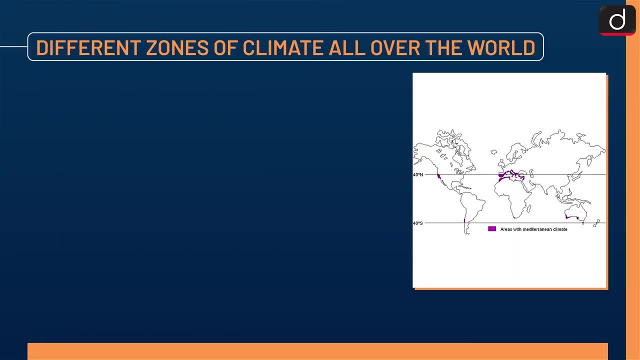 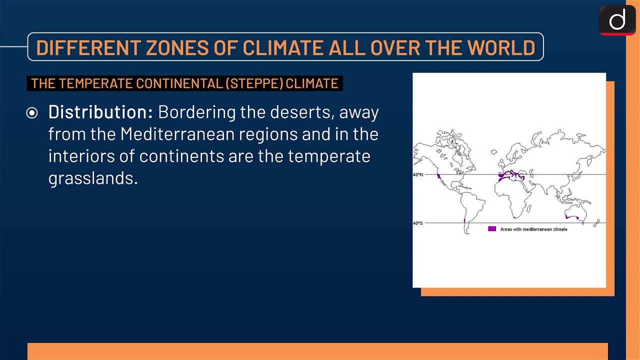 mediterranean lands. next zone is the temperate continental, steepy climate shifting towards the distribution bordering the deserts, away from the mediterranean regions and in the interiors of continents, are the temperate grasslands. in the northern hemisphere the grasslands are far more. 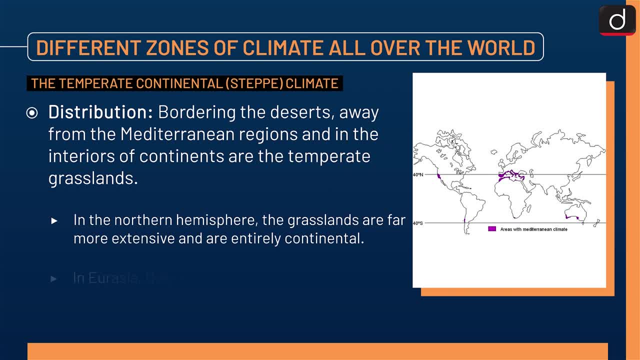 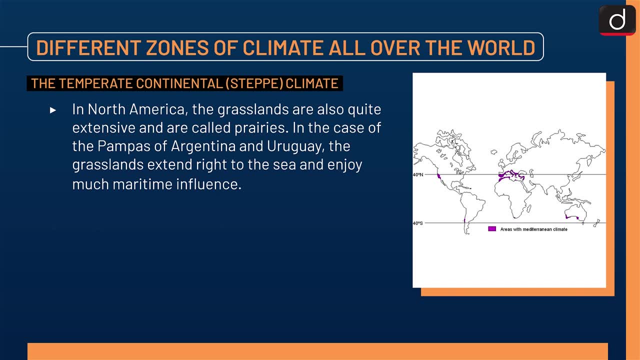 extensive and are entirely continental. in eurasia they are called the steeps. in north america the grasslands are also quite extensive and are called prairies. in the case of the pampas of argentina and irugway, the grassland tend right to the sea and enjoy much maritime influence. in south africa the grasslands are 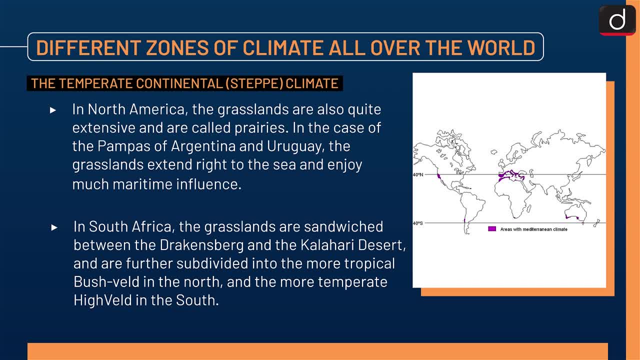 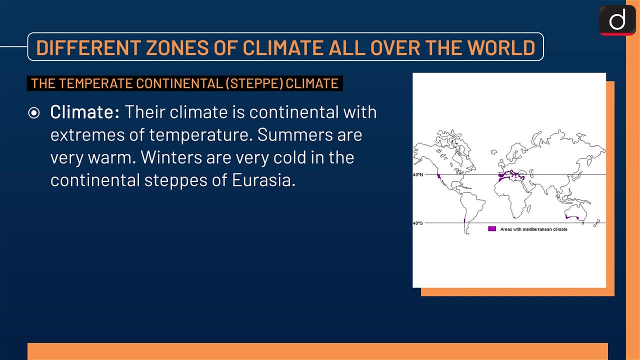 sandwiched between the drakensberg and the kadahari desert and are further subdivided into the more tropical bush weld in the north and the more temperate high weld in the south. next is climate. their climate is continental, with extremes of temperature. summers are very warm, winters are. 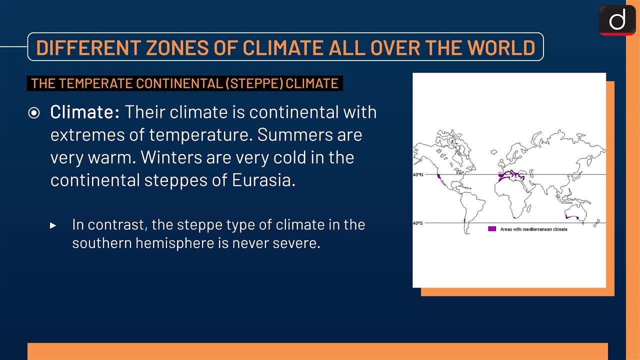 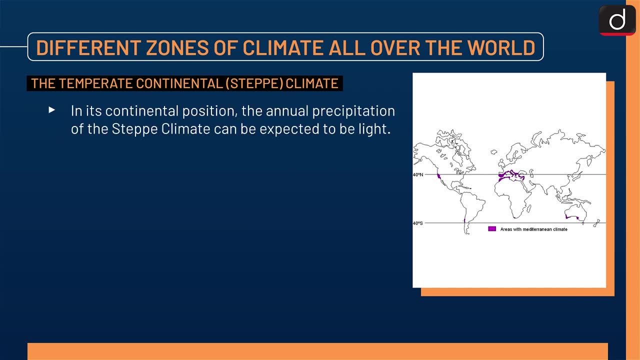 usually the best for the climate of eurasia. in contrast, the steepy type of climate in the southern hemisphere is never severe. the annual range of temperature is great, a direct result of continality in its continental position. the annual precipitation of the steppy climate can be expected. 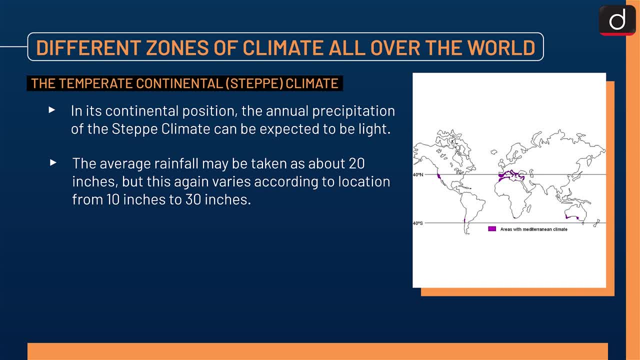 to be light. the average rainfall may be taken as about 20 inches, but this again varies according to 10 inches to 30 inches. natural vegetation: the term steepy vegetation geographically refers to the scanty vegetation of the sub-arid lands of continental eurasia, their greatest difference. 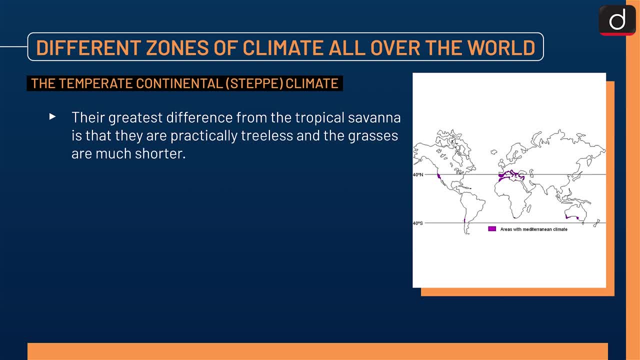 from the tropical savannah is that they are practically treeless and the grasses are much shorter. where the rainfall is moderate, above 20 inches, the grasses are tall, fresh and nutritious: ribed as long prairie grass. next is economy. the temperate grasslands were once the home of grazing. 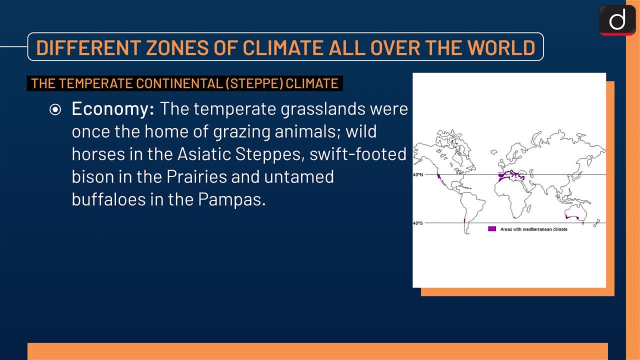 animals: wild horses in the asiatic steeps, swift-footed bison in the prairies and untamed buffaloes in the pampas. even as recently as the last century, these grasslands were dominated by nomadic and semi-nomadic peoples, like the kirghiz of the asiatic steeps, the grasslands. 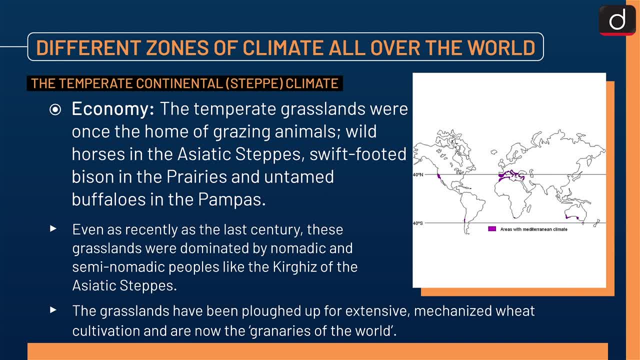 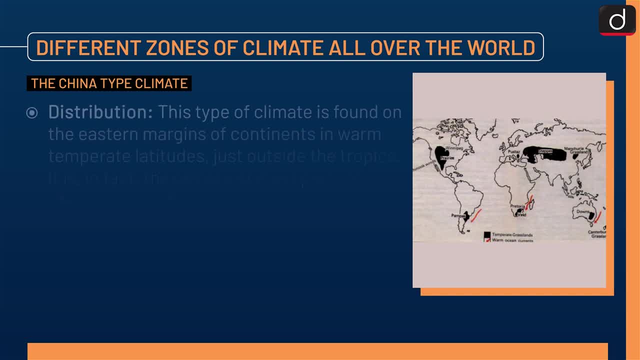 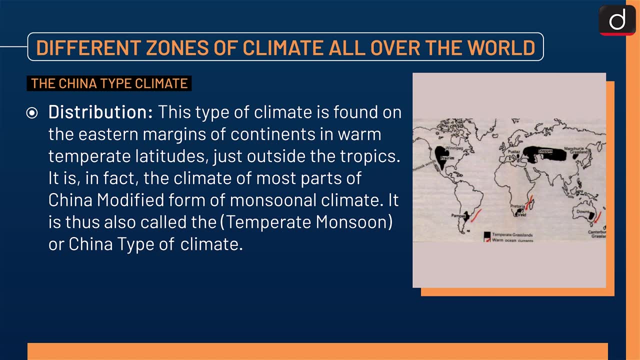 have been plowed up for extensive mechanized wheat cultivation and are now the granaries of the world. next is the China type climate. first of all, distribution. this type of climate is found on the eastern margins of continents, in warm temperate latitudes just outside the tropics. it is in fact 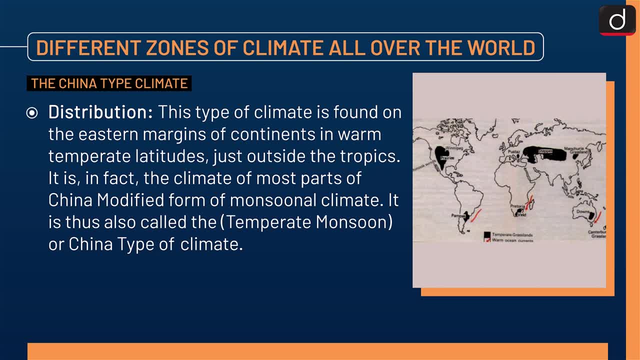 the climate of most parts of China modified form of monsoonal climate. it is thus also called the temptationed monsoons climate, theờ gao climate. the layer of woody atmosphere can form могoulda melt or China type of climate. it is sometimes referred to as the Gulf type of climate. 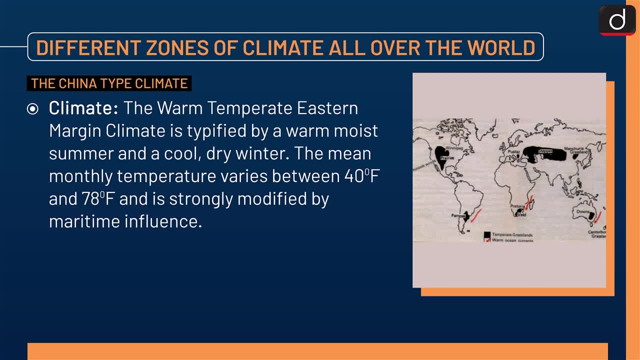 next is climate. the warm, temperate eastern margin climate is typified by a warm, moist summer and a cool, dry winter. the mean monthly temperature varies between 40 degree Fahrenheit and 78 degree Fahrenheit and is strongly modified by maritime influence. the relative humidity is a little high in 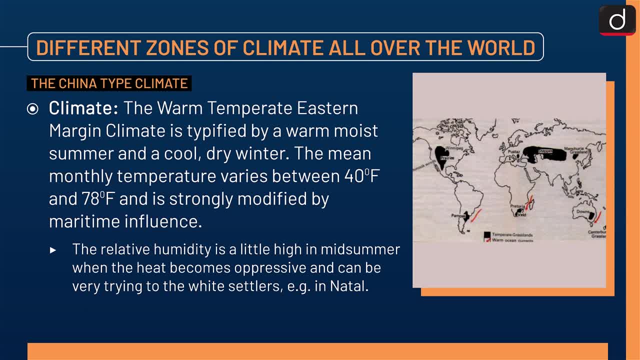 the midsummer when the heat becomes oppressive and can be very trying to the white settlers. example in the natural rainfall is more than moderate, anything from 25 inches to 60 inches. the warm, temperate eastern margin climate supports a wide range of crops. important feature is the fairly uniform 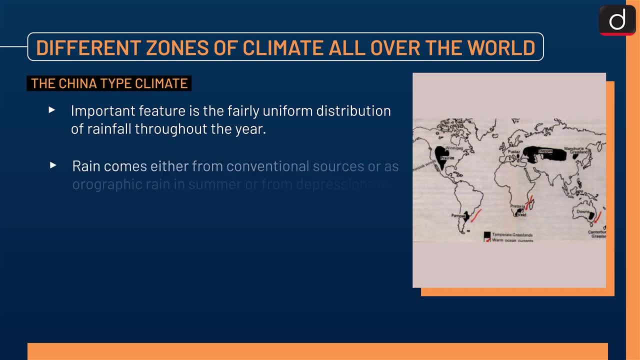 distribution of rainfall throughout the year. rain comes either from conventional sources or as orographic rain, in some cases summer, or from depressions in prolonged showers in the winter. local storms- example typhoons and hurricanes- also occur. next is natural vegetation. the eastern margins of warm, temperate latitude have a much heavier rainfall. 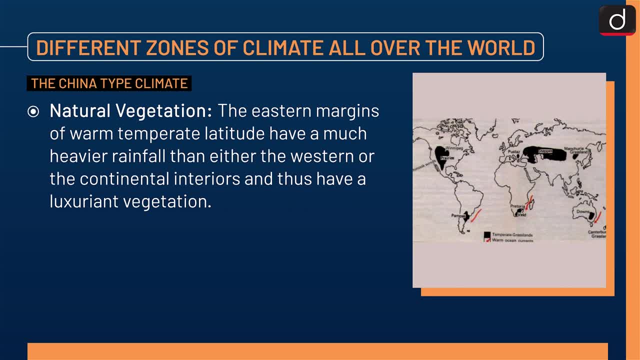 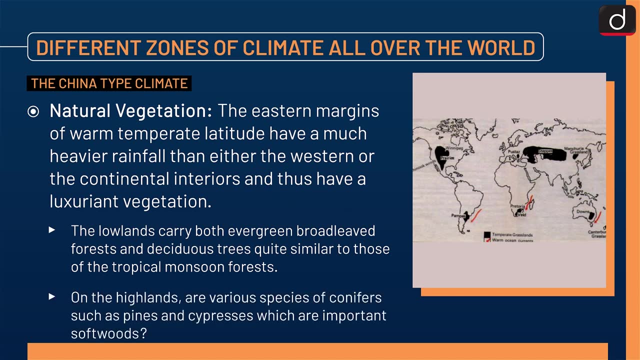 than either the western or the continental interiors, and does have a luxuriant vegetation. the lowlands carry both evergreen broad-leaved forests and deciduous trees, quite similar to those of the tropical sun forest. on the highlands are various species of confers such as pines and 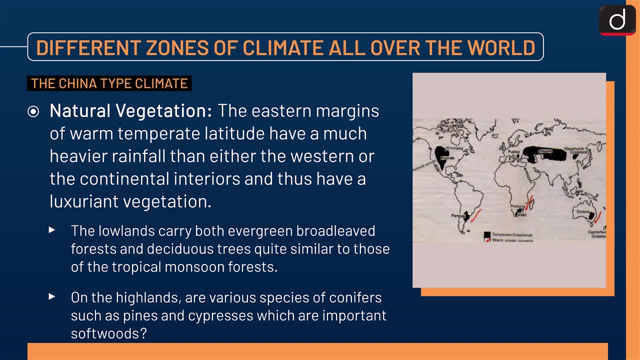 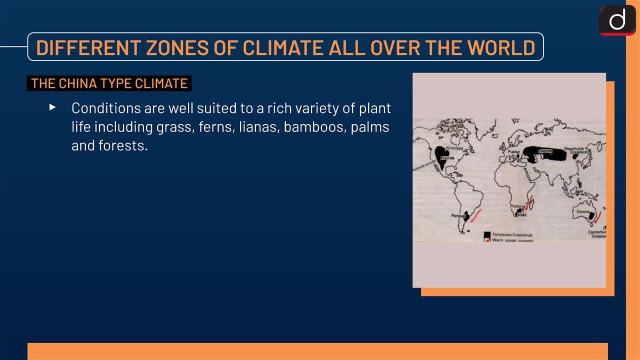 cypresses, which are important softwoods. conditions are well suited to a rich variety of plant life, including grass, ferns, lianas, bamboos, palms and forests. the well distributed rainfall all the year round makes the regions look green at all times. next is economy: the warm temperature. 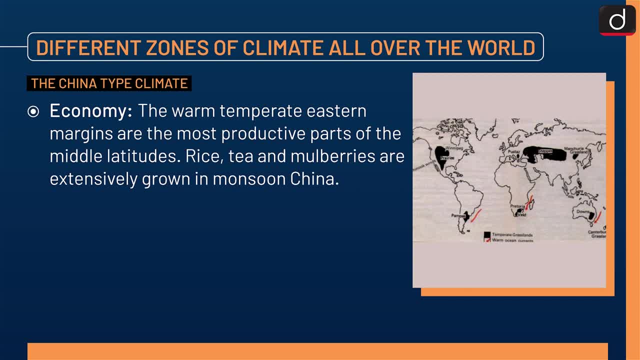 temperate eastern margins are the most productive parts of the middle latitudes. rice, tree and mulberries are extensively grown in monsoon China. elsewhere are found other products of economic importance. example: cane sugar in natal coffee and maize in South America and daring in New South Wales and Victoria. 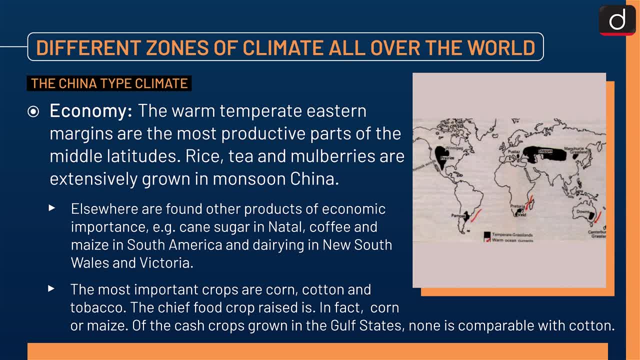 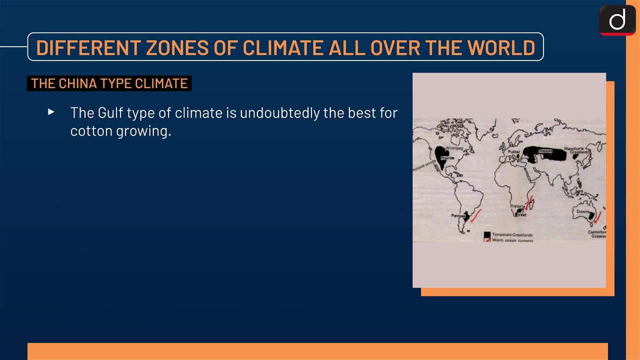 the most important crops are corn, cotton and tobacco. the chief food crop raised is, in fact, corn, cotton and tobacco. the chief food crop raised is, in fact, corn or maize. of the cash crops grown in the Gulf states, none is comparable with cotton. the Gulf type of climate is undoubtedly the best for cotton growing. 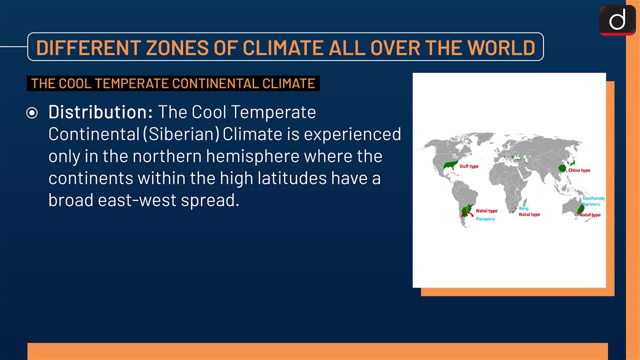 next zone is the cool temperate continental climate. first of all, distribution, the cool temperate continental or Siberian climate is experienced only in the northern hemisphere, where the continents within the high latitudes have a broad east-west spread. on its poleward side it merges into the Arctic tundra of Canada and 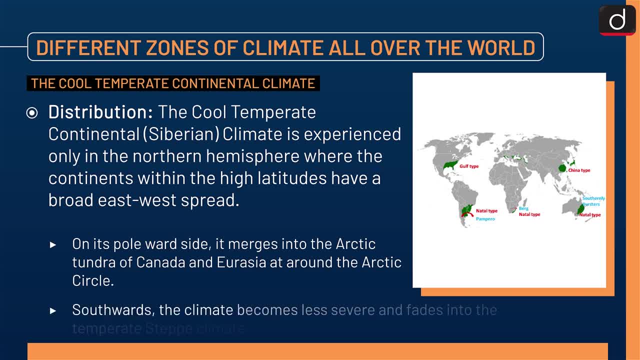 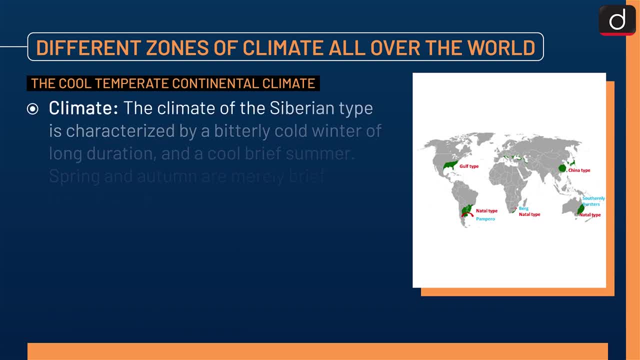 Eurasia, at around the Arctic Circle. southwards, the climate becomes less severe and fades into the temperate, steppy climate. next is climate. the climate of the Siberian type is characterized by a bitterly cold winter of long duration and a cool, brief summer. spring and autumn are nearly brief. 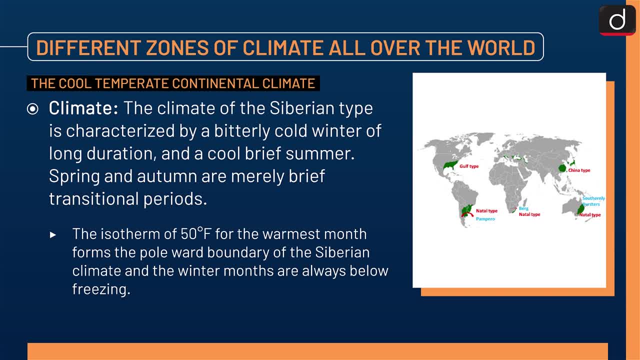 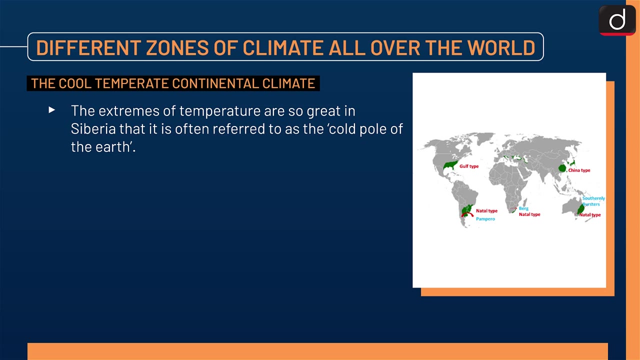 transitional periods. the isotherm of 50-degree Fahrenheit for the warmest month forms the poleward boundary of the Siberian climate, and the winter months are always below freezing. an annual range of 54 degrees Fahrenheit is common in the Siberian type of climate. the extremes of temperature are so great in Siberia that it is often 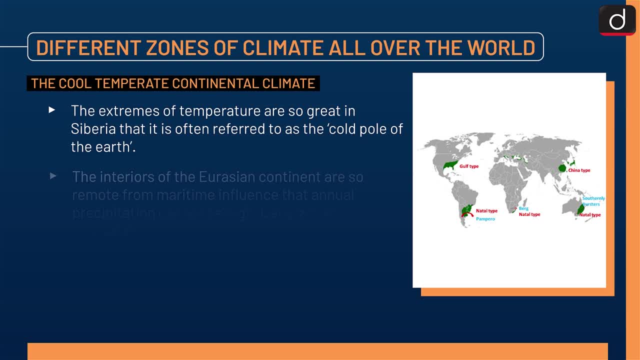 referred to as the cold pole of the Earth. the interiors of the Eurasian continent are so remote from the Father Earth that they can't be crossing the maritime influence that annual precipitation cannot be high. generally speaking, a total of 15 to 25 inches is typical of the annual precipitation of 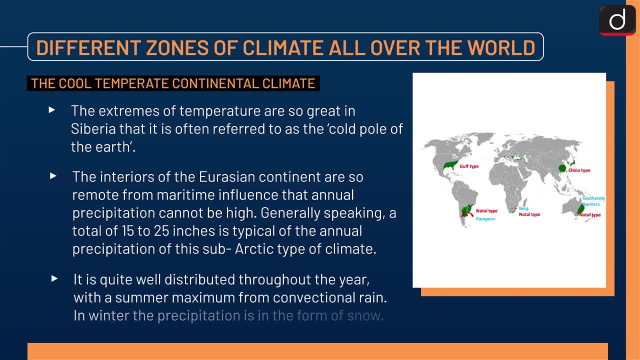 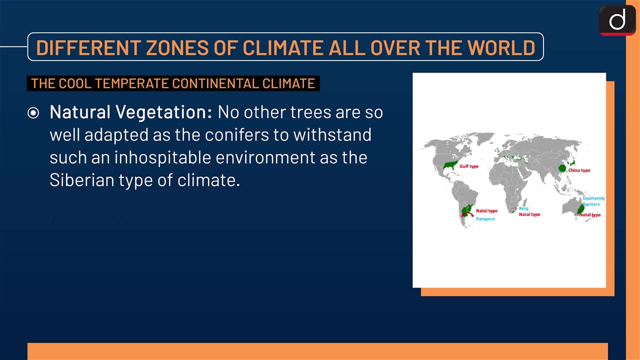 the subarctic type of climate. it is quite well distributed throughout the year, with a summer maximum from conventional rain. in winter the precipitation is in the form of snow. next is natural vegetation. no other trees are so well adapted as the confers to withstand, such as an. 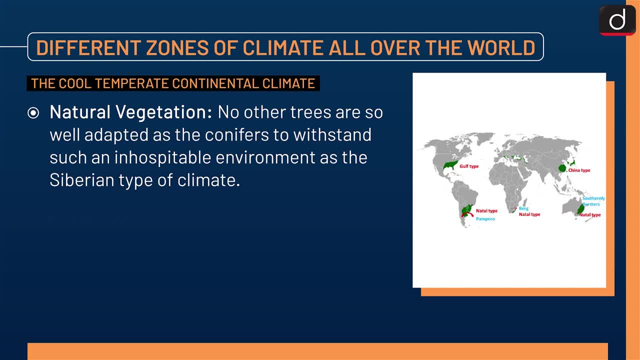 inhospitable environment as the Siberian type of climate. the coniferous forest belts of Eurasia and North America are the richest sources of softwood. the world's greatest softwood producers are the USSR, USA, Canada and the Panoskandian countries. next is economy. the coniferous forest regions of the 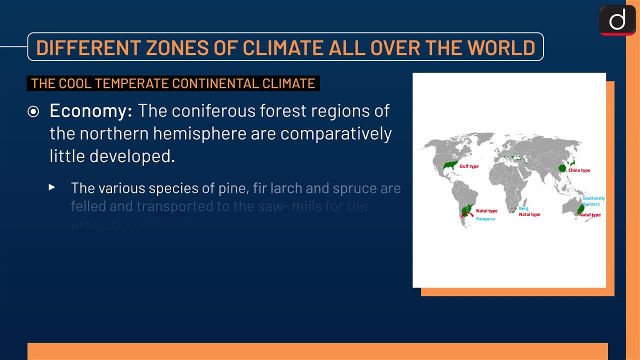 Northern Hemisphere are the most rich in softwood and the largest in the hemisphere, are comparatively little developed. the various species of pine for large and spruce are felled and transported to the sawmills for the extraction of temperate softwoods. there is little agriculture as few crops can. 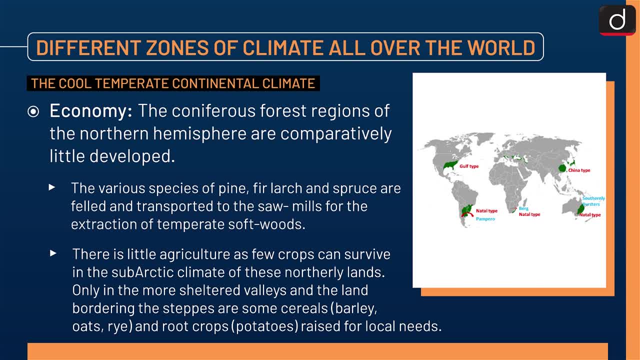 survive in the subarctic climate of these northerly lands only in the more sheltered valleys and the land bordering the steepest are some cereals, barley oats, rye and root crops such as potatoes, raised for local needs. many of the Samoan aids 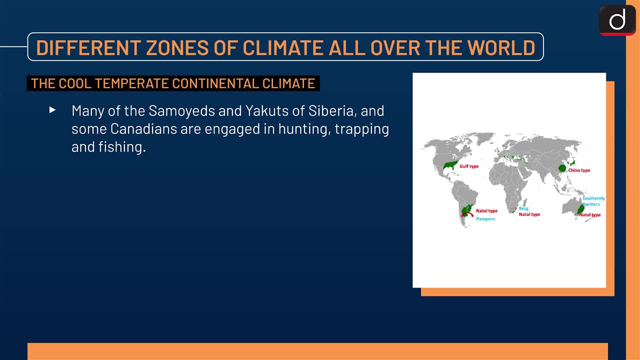 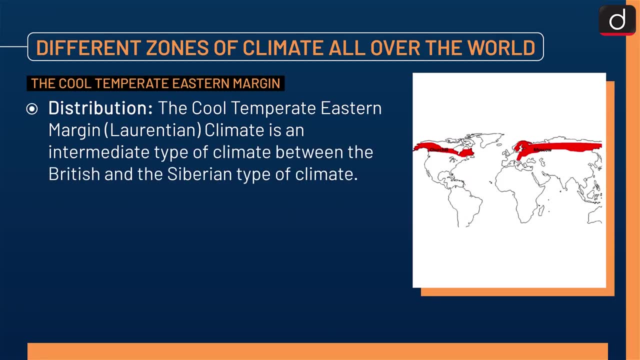 and your goods of Siberia, and some Canadians are engaged in hunting, trapping and fishing. next zone is the cool temperate eastern margin. moving on to the distribution, the cold temperate eastern margin, or Laurentian climate, is an intermediate type of climate between the British and the Siberian type of 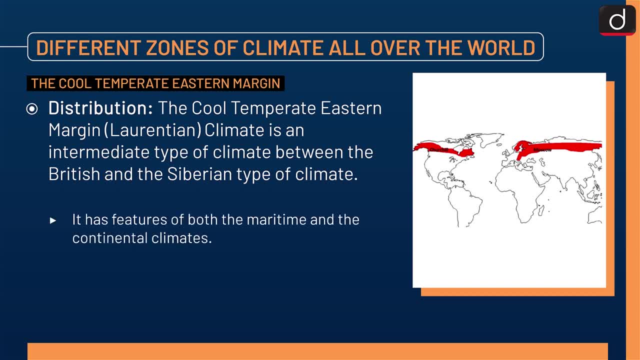 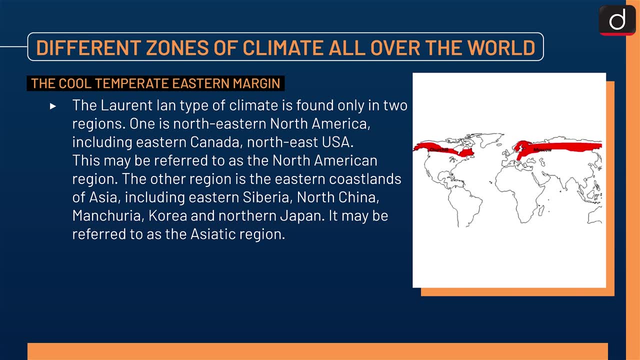 It has features of both the maritime and the continental climates. The Laurentian type of climate is found only in two regions. One is northeastern North America, including the eastern Canada, northeast USA. This may be referred to as the North American region. The other region is the eastern coastlands of Asia, including eastern Siberia. North 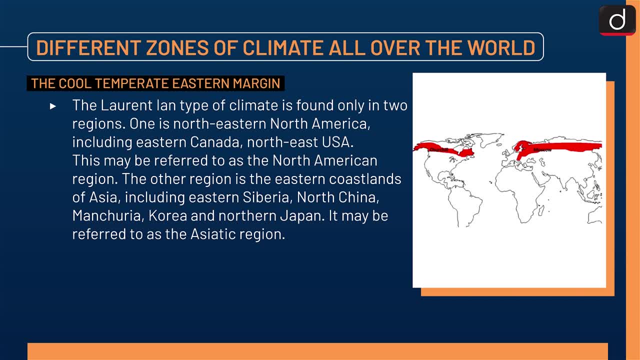 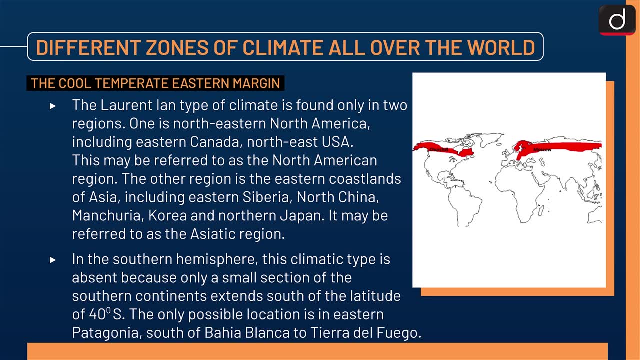 China, Manchuria, Korea and northern Japan. It may be referred to as the Asiatic region In the southern hemisphere. this climatic type is absent because only a small section of the southern continent extends south of the latitude of 40 degrees south. 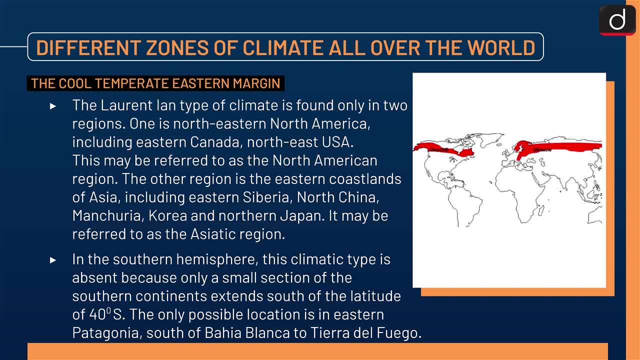 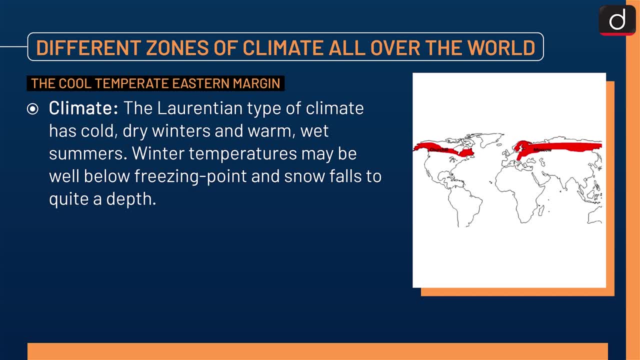 The only possible location is in eastern Patagonia, south of Bahia Blanca to Tierra del Fuego. Next is climate. The Laurentian type of climate is found only in two regions. The northern climate has cold, dry winters and warm, wet summers. 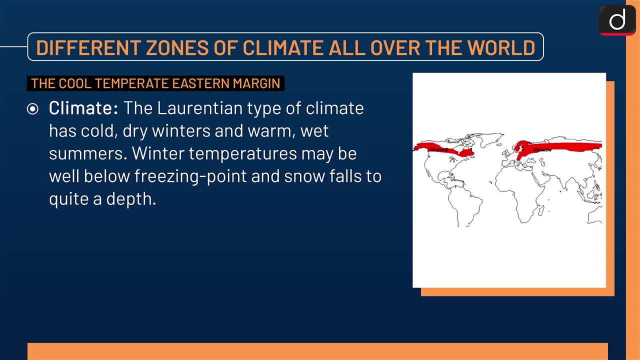 Winter temperatures may be well below freezing point and snow falls to quite a depth. Summers are as warm as the tropics, ie 70° to 80° F. Though rain falls throughout the year, there is a distinct summer maximum from the easterly winds, from the oceans. 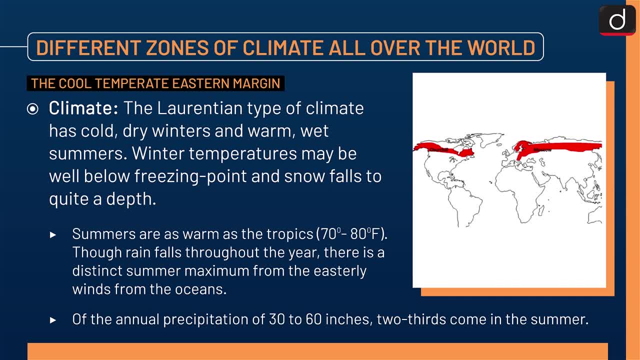 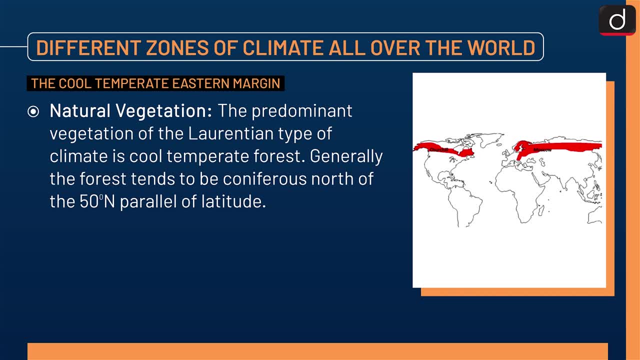 Of the annual precipitation of 30 to 60 inches, two-thirds come in the summer. In the northern hemisphere, the Laurentian type of climate is found only in two regions. Next is natural vegetation. The predominant vegetation of the Laurentian type of climate is full temperate forests. 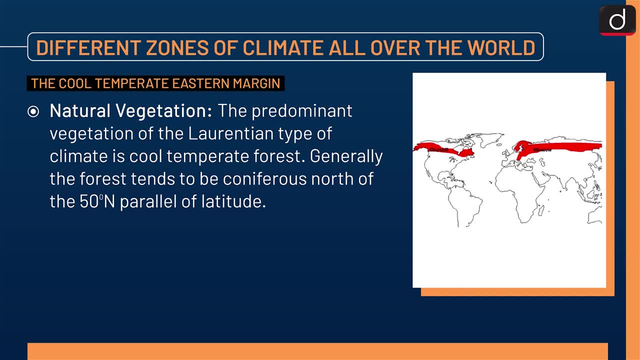 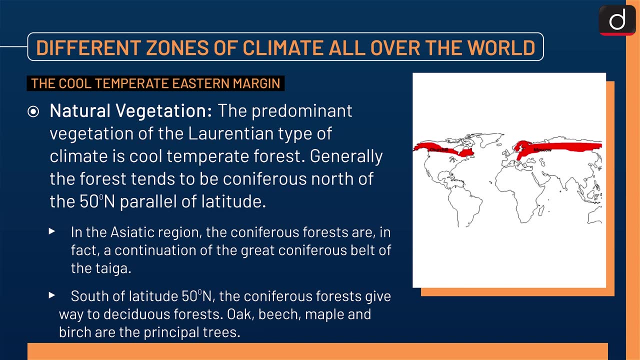 Generally, the forest tends to be coniferous north or 50° North parallel of latitude. In the Asiatic region, the coniferous forests are in fact a continuation of the great coniferous belt of the Taiga. South of latitude, 50° North, the coniferous forests give way to deciduous forests. 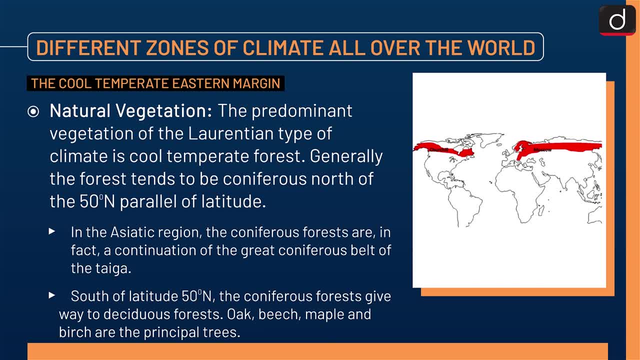 Theides of the Asiatic region give way to deciduous forests. The coniferous forests give way to deciduous forests. Theides of the Asiatic region give way to deciduous forests. oak beech, maple and birch are the principal trees. 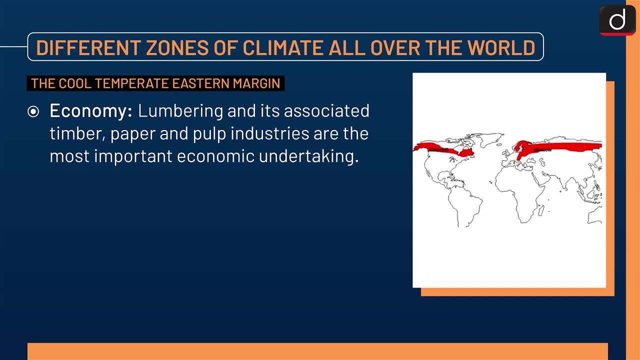 Next is economy. Lumbering and its associated timber, paper and pulp industries are the most important economic undertakings. Lumbering has always been a major occupation of this sparsely populated part of eastern Asia, and timber is a leading export item. 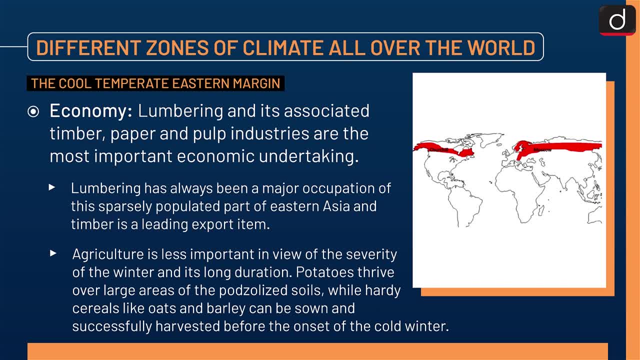 Agriculture is less important in view of the severity of the winter and its long duration. Rotators thrive over large areas of porzolized soils, while the hardy cereals like oats and barley can be sown and successfully harvested before the onset of the cold winter. 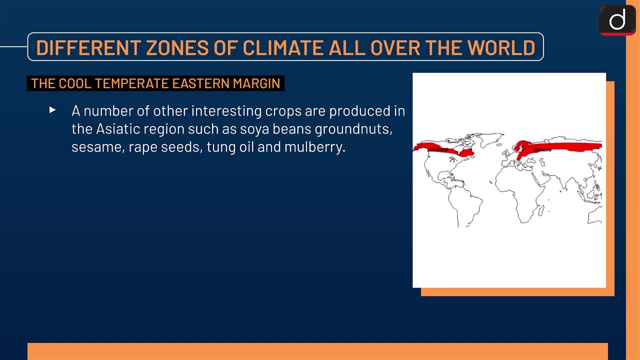 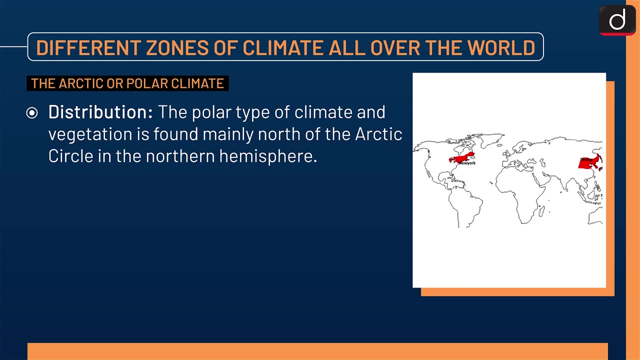 A number of other interesting crops are produced in the Asiatic region, such as soya beans, groundnuts, sesame, rapeseed, tung oil and mulberry. Next zone is the Arctic Or polar climate, Shifting towards the distribution, the polar type of climate and the vegetation is found in mainly. 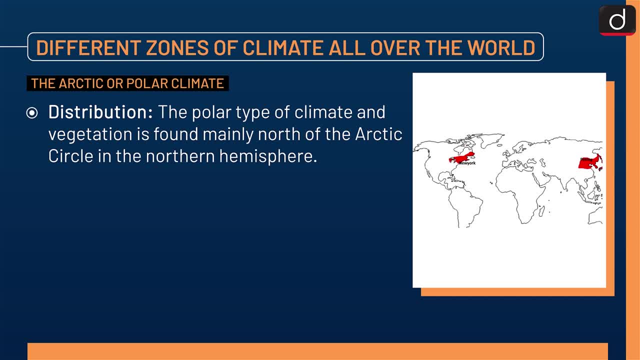 north of the Arctic Circle. in the northern hemisphere, The ice caps are confined to green land and to the highlands of these high latitude regions, where the ground is permanently snow covered. The lowlands, with a few months ice free, have tundra vegetation. Next is climate. 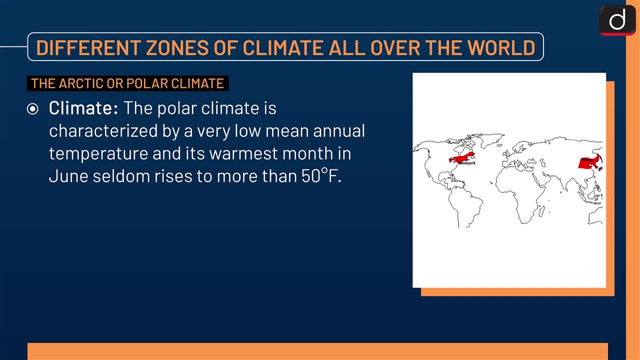 The polar climate is characterized by a very low mean of annual temperature, and its warmest month, in June, seldom rises to more than 50 degrees Fahrenheit. Winters are long and very severe. Summers are cool and brief. At the North Pole, there are six months without light in winter. 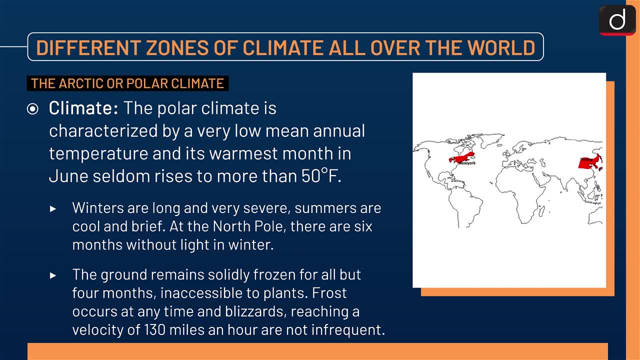 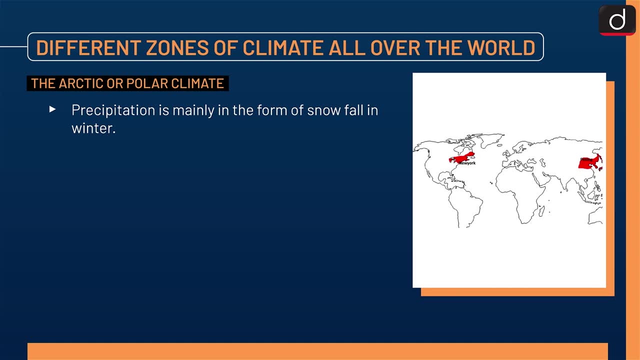 The ground remains solidly frozen for all but four months, inaccessible to plants. Frost occurs at any time and blizzards reaching a velocity of 130 miles an hour are are not infrequent. precipitation is mainly in the form of snow falling in winter. next is natural vegetation in such an adverse environment as the. 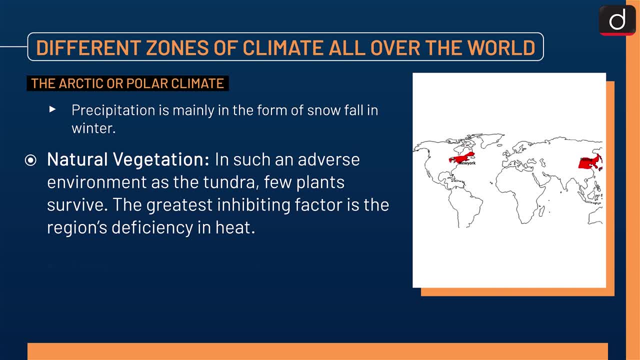 tundra, few plants survive. the greatest inhibiting factor is the region's deficiency in heat. there are no trees in the tundra. such an environment can support only the lowest form of vegetation: mosses, lichens and sedges. next is economy. human activities of the tundra are highly confined to the coast. 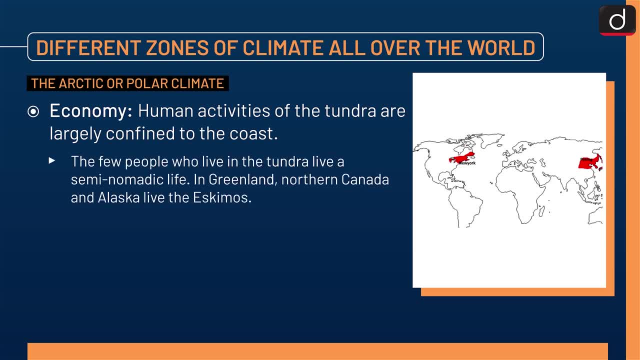 the few people who live in the tundra live in a semi nomadic life. in Greenland, northern Canada and Alaska live the Eskimos. they used to live as hunters, fishers and food gatherers. during winter they live in compact igloos and in summer they have to live in a netherland. 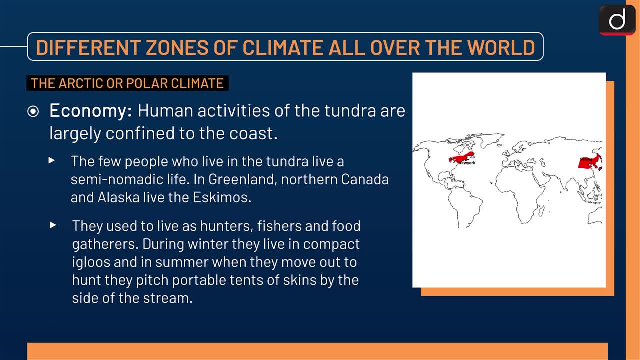 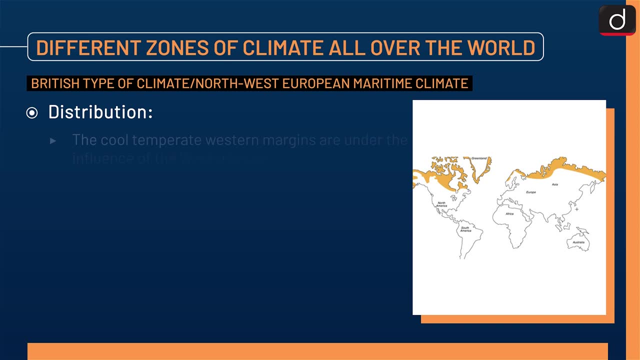 When they move out to hunt, they pitch portable tents of skins by the side of the stream. Their food is derived from fish, seals, walruses and polar bears. Now the last zone we are going to discuss is British type of climate or North West European. 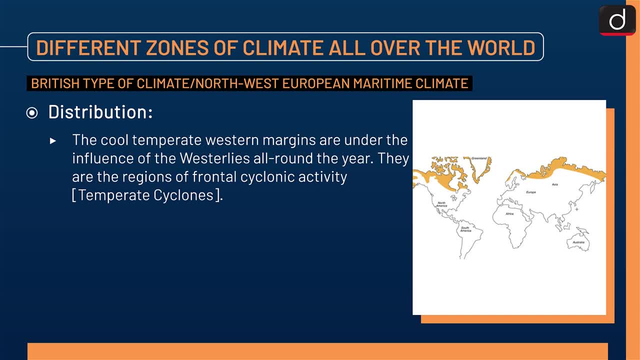 maritime climate. Moving on to the distribution, the cool, temperate western margins are under the influence of the Westerlies all round the year. They are the regions of frontal cyclonic activity, like temperate cyclones. This type of climate is typical to Britain, hence the name British type, also called as 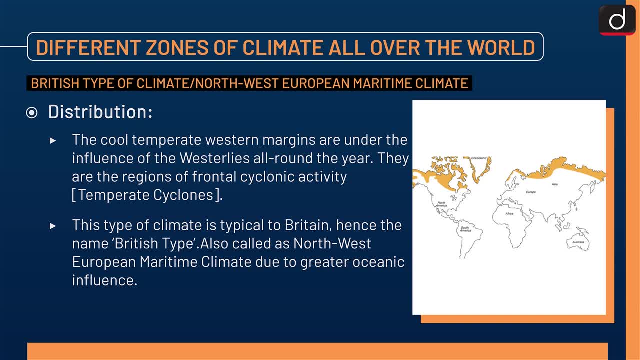 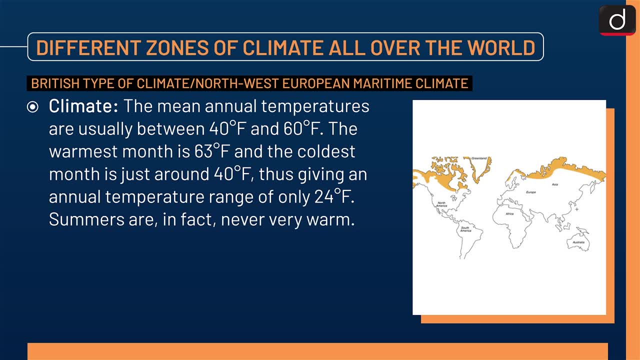 North West European maritime climate due to greater oceanic influence. Next is climate. The mean annual temperatures are usually between 40 degree Fahrenheit and 60 degree Fahrenheit. The warmest month is 63 degree Fahrenheit and the coldest month is 20 degree Fahrenheit. 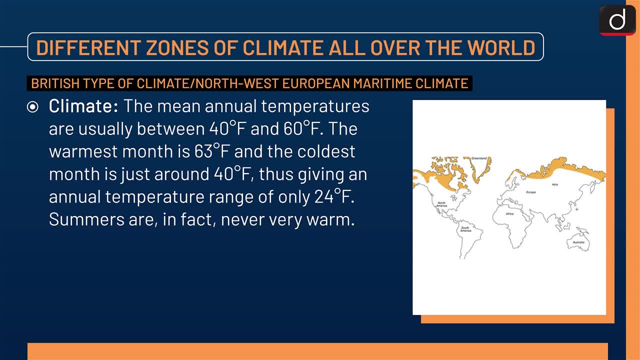 Thus giving an annual temperature range of only 24 degree Fahrenheit. Summers are, in fact, never very warm. The climate is ideal for maximum comfort and mental alertness. Winters are abnormally mild. The British type of climate has adequate rainfall throughout the year, with a tendency towards 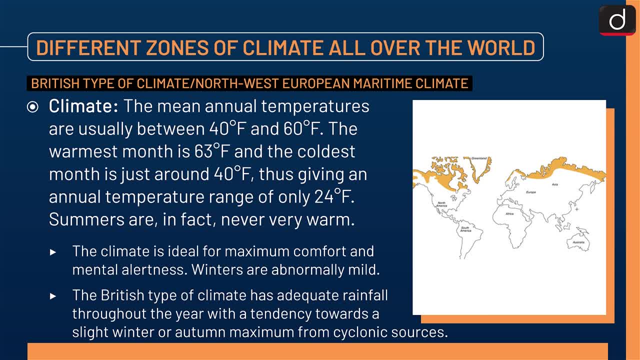 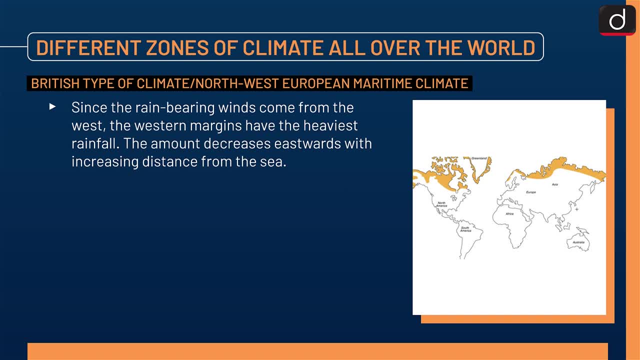 a slight winter or autumn maximum from cyclonic sources. Since the rain-bearing winds tend to be very mild in the winter, the average temperature is around 40 degree Fahrenheit. The most common rainfalls come from the west. The western margins have the heaviest rainfall. 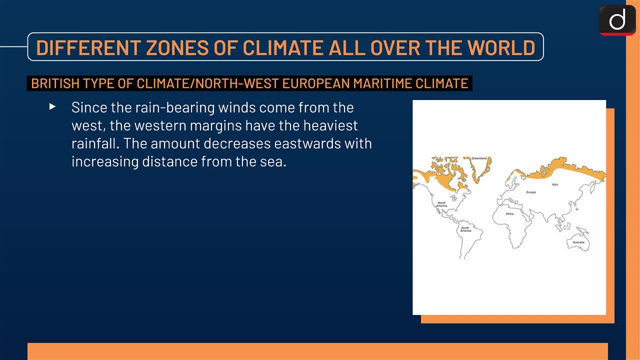 The amount decreases eastwards with increasing distance from the sea. Next is Natural Vegetation. The natural vegetation of this climate time is deciduous forest. Some of the more common species include Oak, Elm, Ash, Birch, Beech, Poplar and Hornbeam. 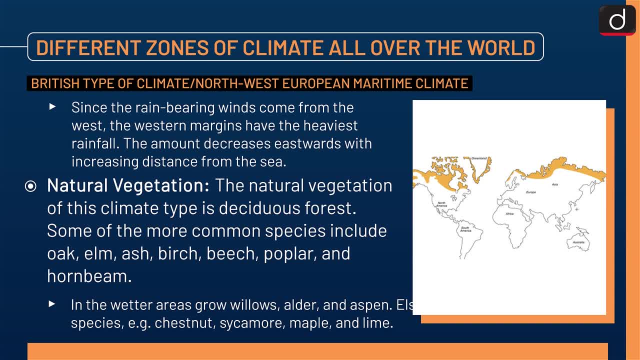 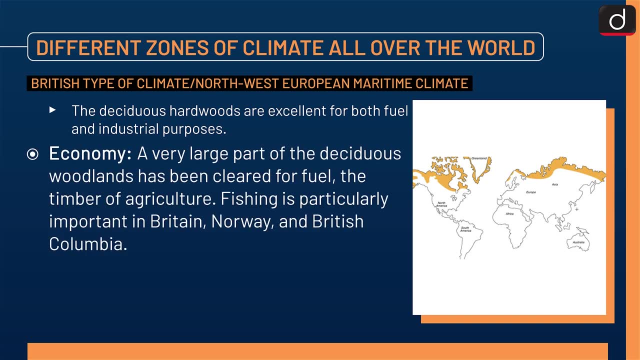 In the wetter areas grow Willows, Alder and Aspen. Elsewhere are found other species, For example Chestnut, Sycamore, Maple and Lime. The deciduous hardwoods are excellent for both fuel and industrial purposes. Now, lastly, Economy. 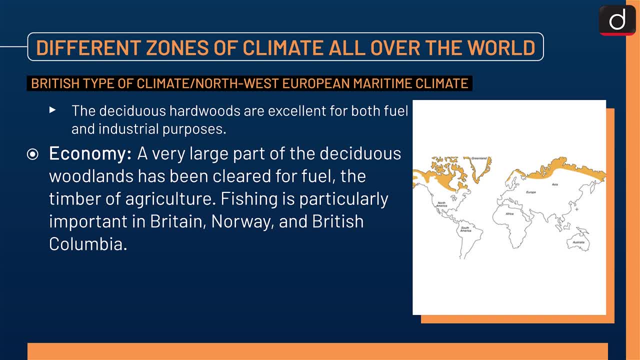 A very large part of the deciduous woodlands has been cleared for fuel, the timber of agriculture. Fishing is particularly important in Britain, Norway and British Columbia. Though market gardening is practiced throughout the world wherever there is a large urban population, nowhere else is it so highly specialized as in Northwest Europe. 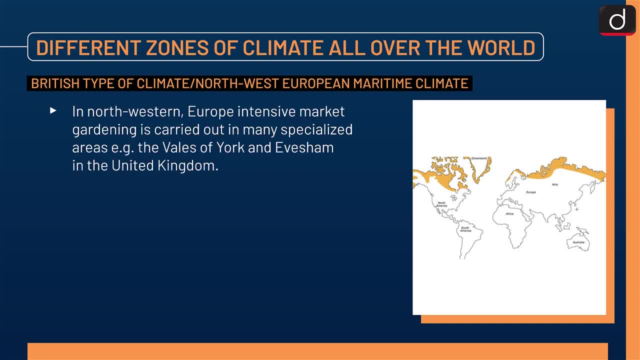 In Northwestern Europe's extensive market gardening is carried out in many specialized areas, For example the Wales of York and Avisham in the United Kingdom. There is no wonder the Australians nicknamed Tasmania the Garden State. So that's all for today. 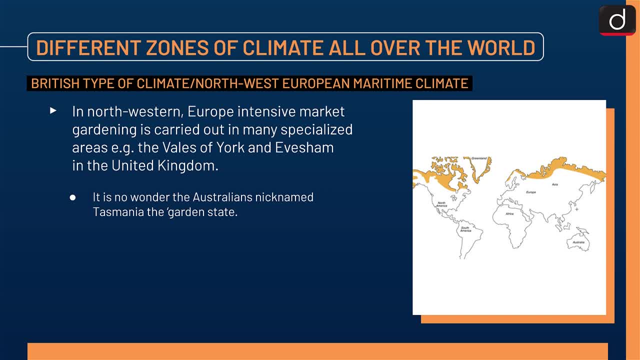 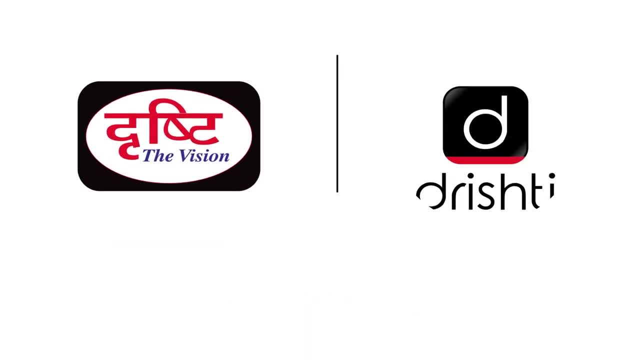 Stay tuned for the next episode. Thanks for watching. I'll see you next time.